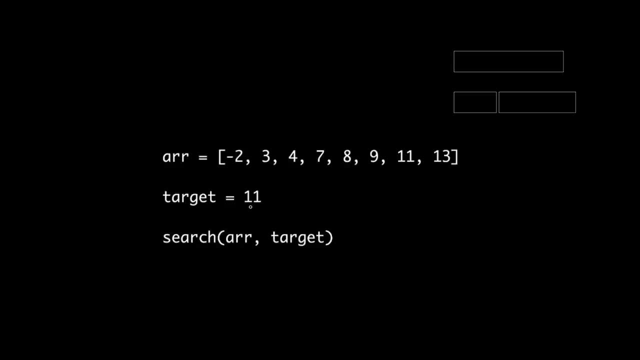 return 6 because the index of the target integer 11.. seven right here is six, And one approach you can use to solve this problem, as a comparison to binary search, is called linear search. The idea of this approach is you start at the beginning of the array, this one right here, and then check if it's our target or 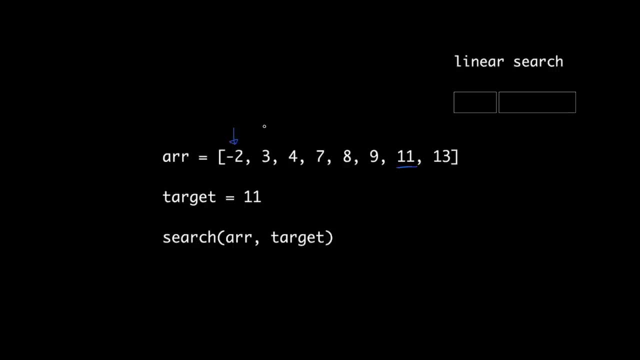 not. And if it's not our target, then we go to the next element, and the next element soon, until we find our target. or we don't find our target but find a number that's larger than the target, Then we can stop the search. then- And this approach has the time complexity- 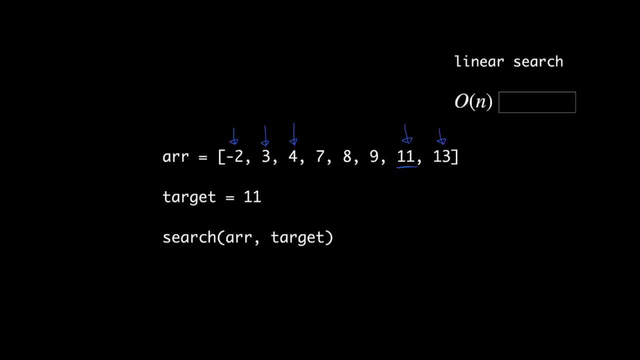 of O, where n is the number of elements in the array. And that's because, assuming that we don't know where the target is, we're going to check a certain number of elements in the array And, on average, we'll need to check about half the elements because, on average, you 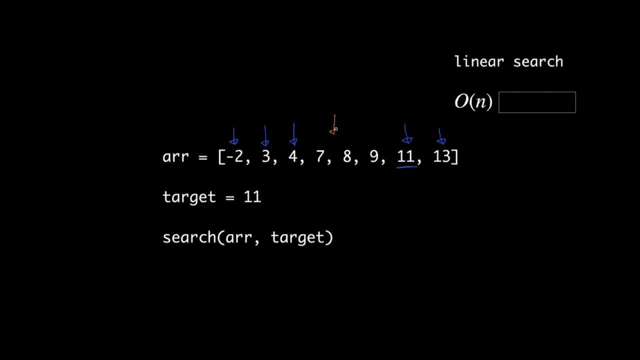 know, we can assume that the target is going to be in the middle of the array, And so we'll need to check n over two elements on average, And that's why we have O in time, which is equivalent to O. Okay, so as a better, faster alternative to linear search, let's: 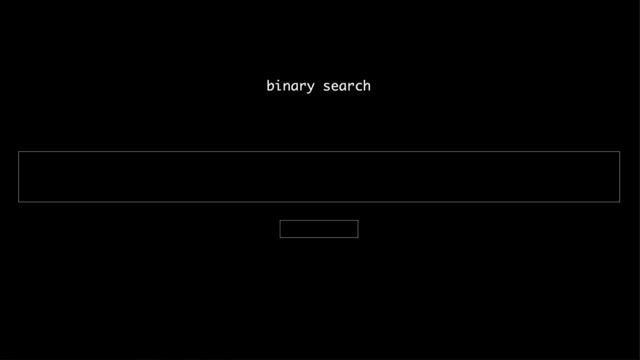 take a look at binary search And to see how it works. we're going to use this example of a sorted array of integers ranging from minus 50 to 50. And, as you can see, we have 40 integers here. We're also 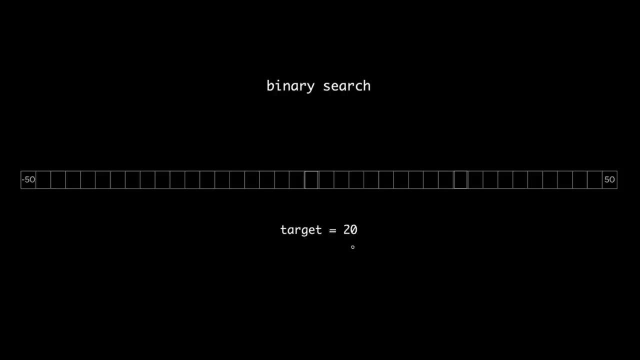 given the integer target of 20.. Now the first step in binary search is to say if the target exists in this array, it must be between the first element and the second element, And the second element is the first element. So this element, right here, and the last element. 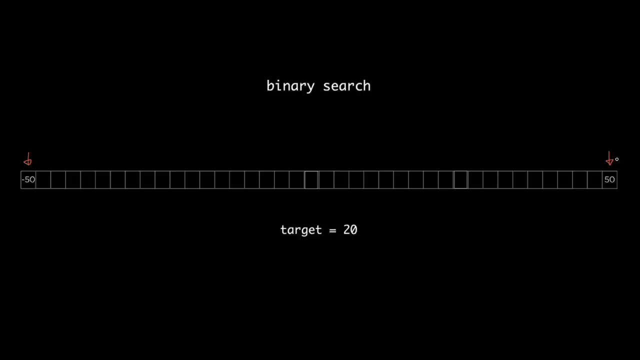 this element right here. Another way to say the same thing would be to say: our initial search region is going to be this entire array which is between the first element and the last element. we can express the idea by defining two integer variables or two pointers which. 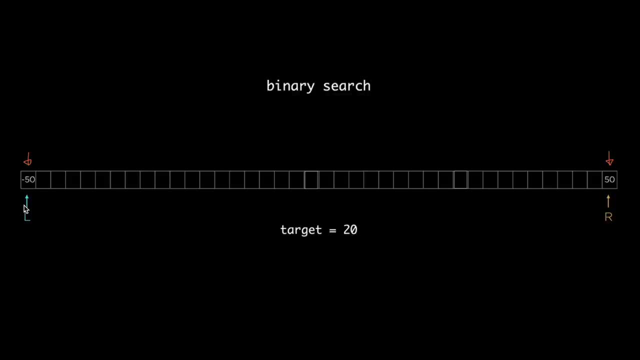 we're going to call left and right or L and R. so L would be zero, pointing at this element right here, and R would be pointing this last element right here, and in this particular example, the initial value of R would be 39 because the length of the array is 40, right here. 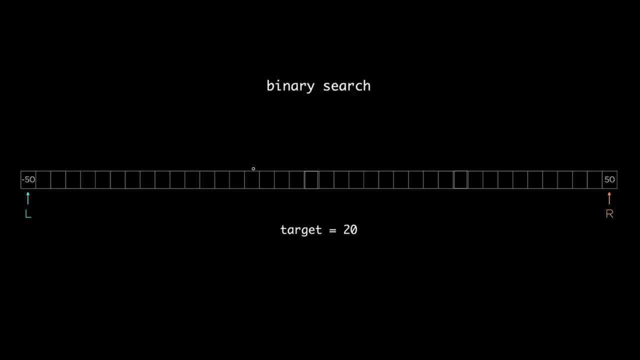 okay, and the next step in binary search would be to check the number that's in the middle of L and R. in this particular case, that's this number right here, and let's say as an example that it happens to be 10. then at that point, since our 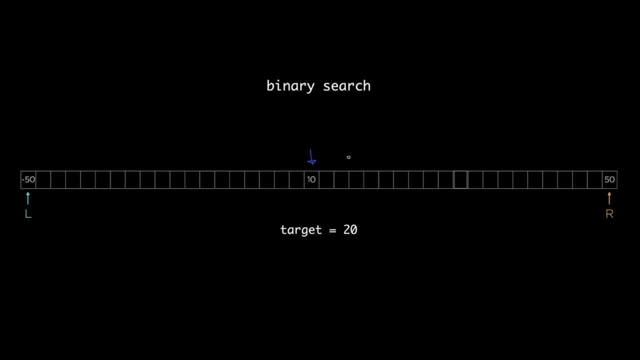 target is larger than 10, we'll know that the target, if it exists in this array, must be in this region right here. so that means we can move our left pointer or L over here, and then we can keep repeating the same procedure to narrow our region. 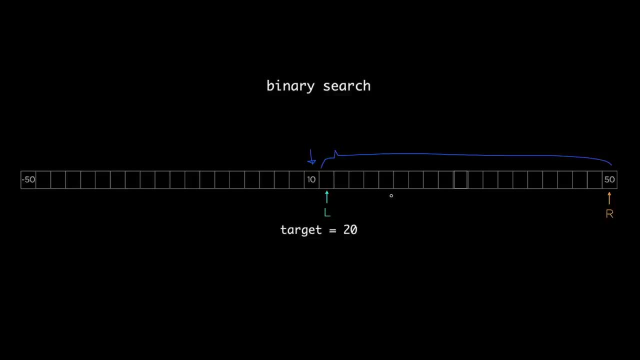 more and more. so we can check the number in the middle of the new value of L and the current value of R. that's this number right here. and if that happens to be larger than target, that's 30, right here. then we'll know our target must be. 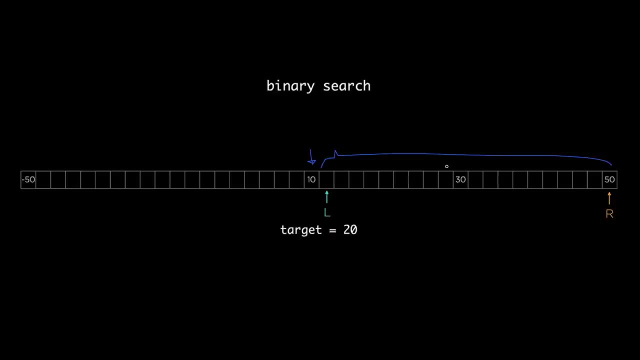 between this current value of L and this element right here. so we can move R over here. so, just like that, we can keep repeating the same procedure until the number between L and R, the number in the middle of L and R, happens to be the target. at that point we can finish running our function because we've already found a. 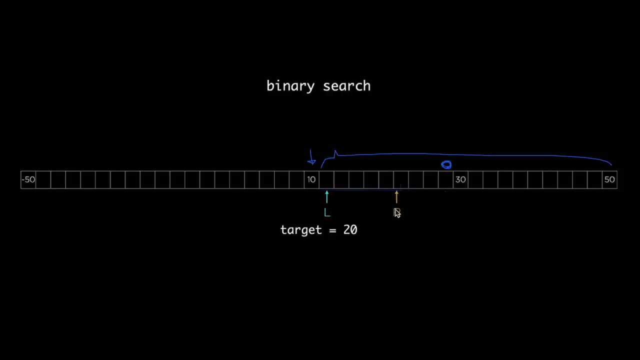 number, or when R comes to the left of L, kind of like that. and that's because at that point our search region is empty, so we may need to move it somewhere else too empty. So that means that this target number doesn't exist in this array. Okay, so we're going. 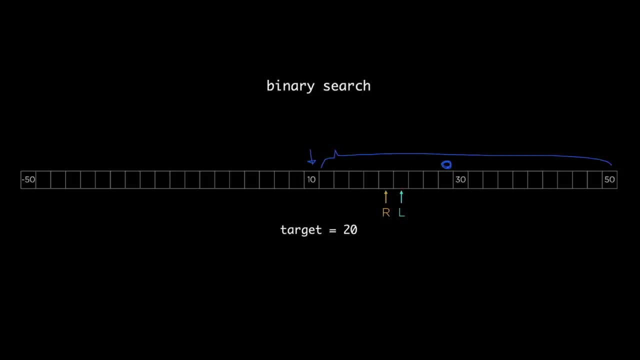 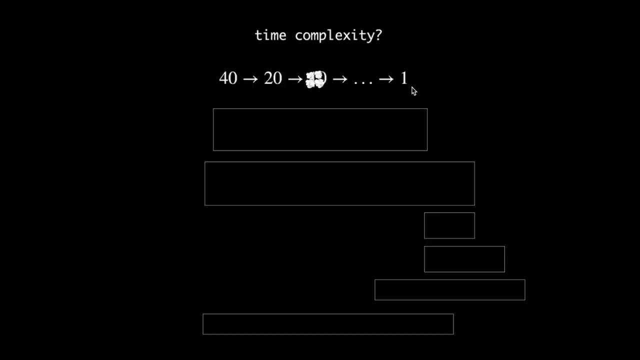 to put this idea into code. But first, before that, let's think about the time complexity of this approach. Well, with this particular example that we just saw, our search region started with 40 elements, and then it became about 20, and then about 10, and so on until we got down to one. 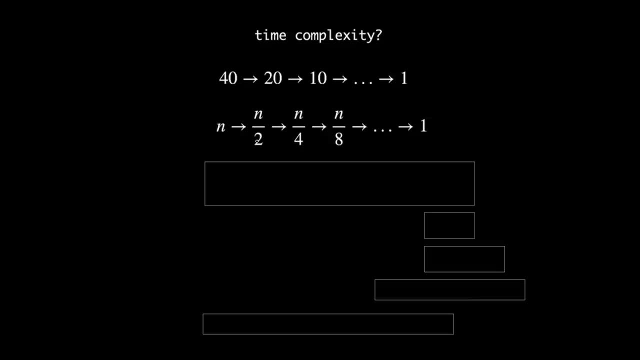 So the pattern we see here is we start with a search region of n elements, which is the number of elements in the given array, And then we half it, and then we get half of that and half of that, and so on, until we get one, And I can write it slightly differently, just like that. So we have 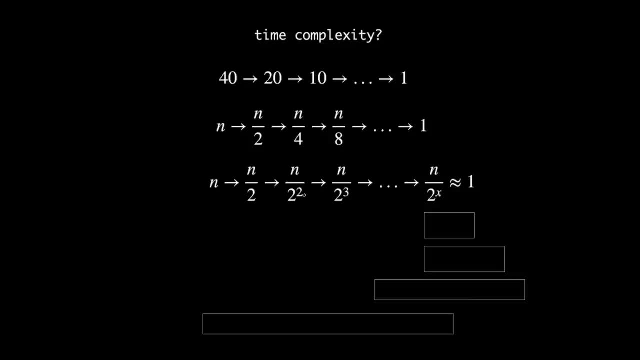 n, and then n over 2, and over 2 to the power of 2, and so on until. And now for a second. let's say that n happens to be 8.. That's 2 to the power of 3.. So this: 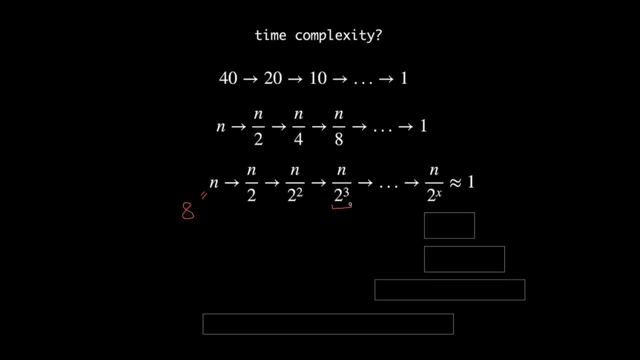 expression right here: n over 2 to the power of 3, becomes 1.. So that means if n happens to be 8, we'll need to check about 3 elements until our search region becomes 1.. You might say: 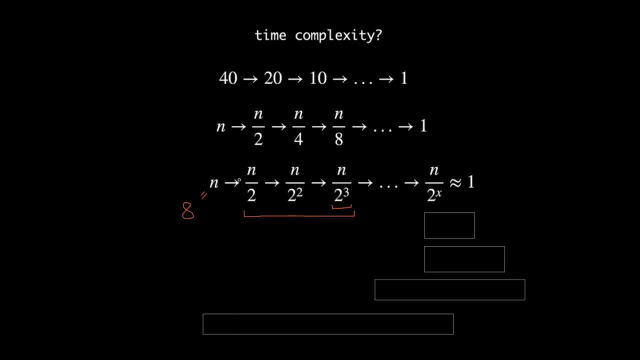 well, that's more like 4 elements, but I'm saying the number of elements that we need to check is roughly equal to 3.. So what I just showed you here is that when n is equal to 2 to the power of 3, we'll need to check about 3 elements for this algorithm to be 1.. So that's 2 to the power of 3.. 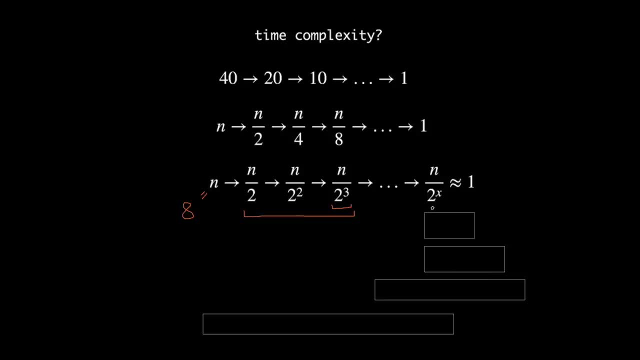 complete. So if n is roughly equal to 2 to the power of x, then we'll need to check about x elements. So, basically, to find the number of elements that we need to check, we only need to find x, such that 2 to the power of x is roughly equal to n. And if you solve this for x, of course. 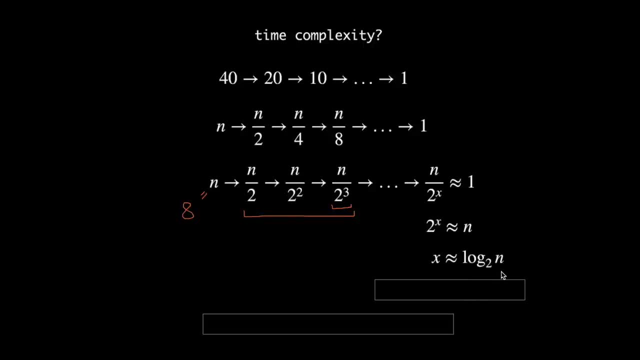 you get x being roughly equal to log 2.. And so the time complexity of this algorithm will be O of the number of elements that we need to check, which is of log 2 of n, And you can rewrite it as of log n, for short. 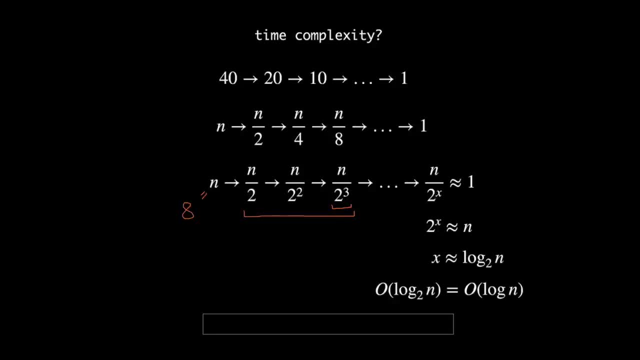 Okay, so what I showed you here is not an exact mathematical proof, But I hope that at least this logic is clear enough to you. Anyway, as an example, if you had 10 million elements in the array, then the number of elements that we need to check will be roughly equal to log 2 of 10. 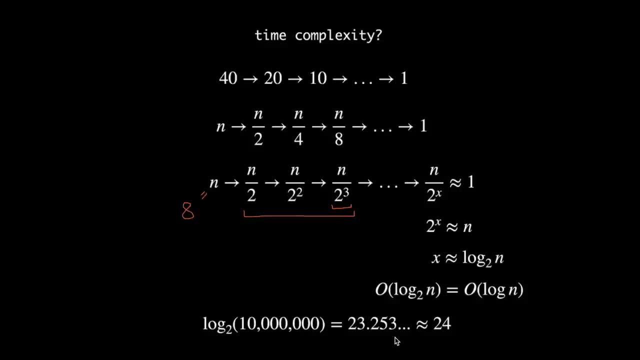 million, which is 23.253, and so on, which is about 24.. So if you had 10 million elements in the given sorted array, you'll need to check at most about 24 elements to find the target number that you're. 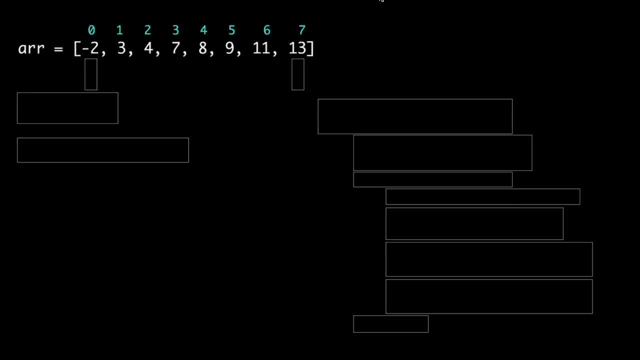 given. Now we're going to put our approach into actual code And to do that, we're going back to our smaller example that we saw earlier. So we're going to put our approach into actual code And to do that, we're going back to our smaller example that we saw earlier. So we're going to put our 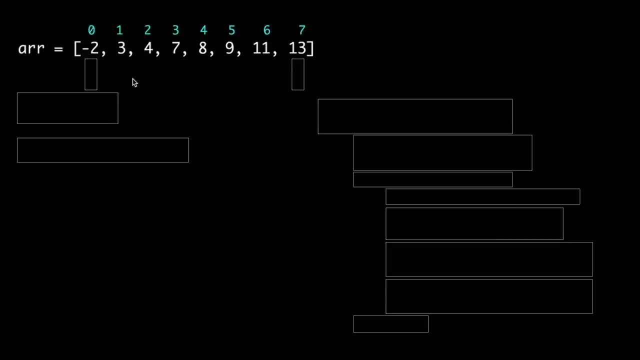 approach into actual code And to do that, we're going back to our smaller example that we saw earlier at the beginning of this video. we just have eight elements in this array And we're also given the at the beginning of this video. we just have eight elements in this array And we're also given the. 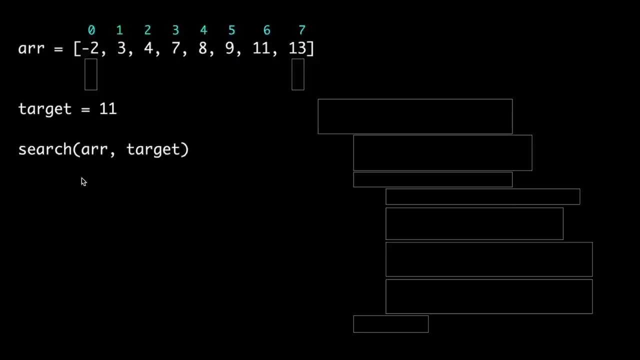 target of, let's say, 11. And we're trying to write our function search that takes these two arguments And, by the way, I'm going to show you some suit code that looks like Python here. but you'll be able to find the actual Python and Java code that I wrote for this at this URL. Anyway, 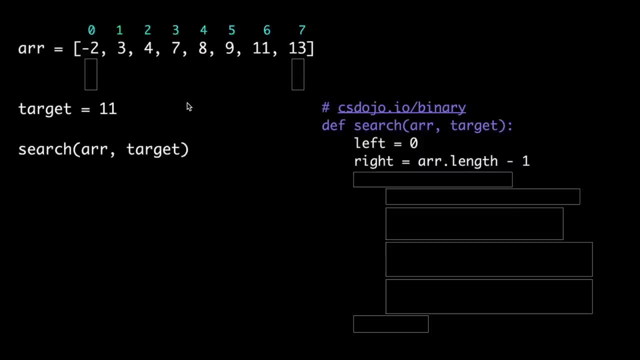 the first step in this code is defining our left and right pointer. Left or L will be 0, right here, and right or R will be the array's length minus 1.. So the array's length is 8 here, and so R will be 7.. And then after that. 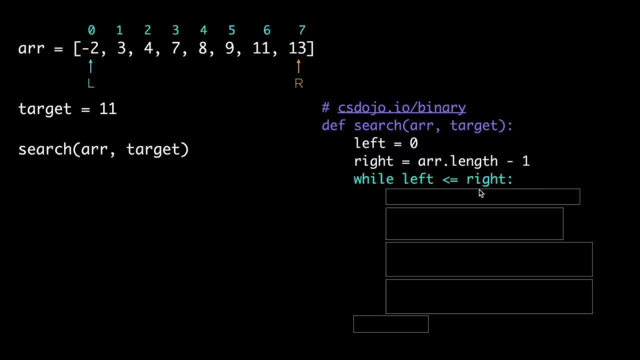 we'll run a while loop saying: while left is less than or equal to right, Or in other words, while right is not to the left of L, And we'll say, while that condition holds, we'll first need to find the mid index, and that's going to be between left and right, And that's going to be. 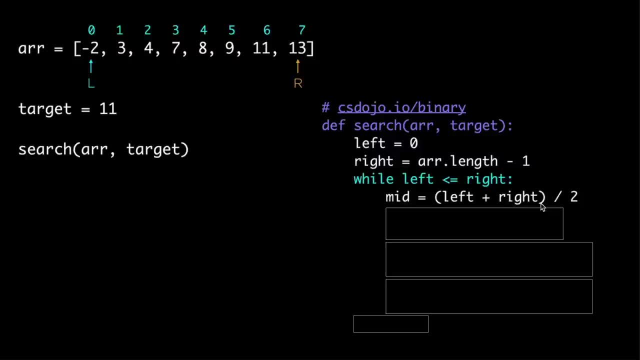 the average of left and right. so left plus right divided by 2.. And if this is not an integer, you can round it down to get an integer value here, And so in this particular example, we'll get 0 plus 7 divided by 2, which is 3.5,. 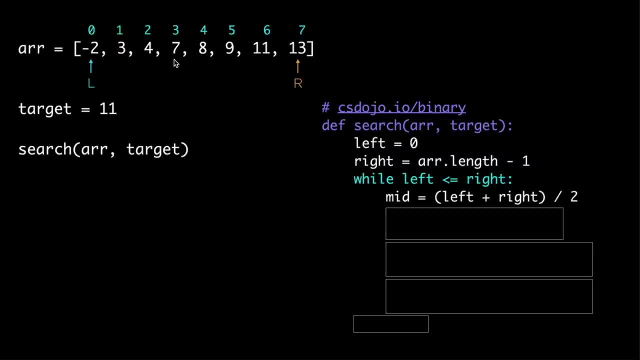 round it down and we get 3.. So mid will be 3 right here, And the next step after that will be to say: if that element R of mid happens to be the target, then we've found the target. So we're going to return that index mid. 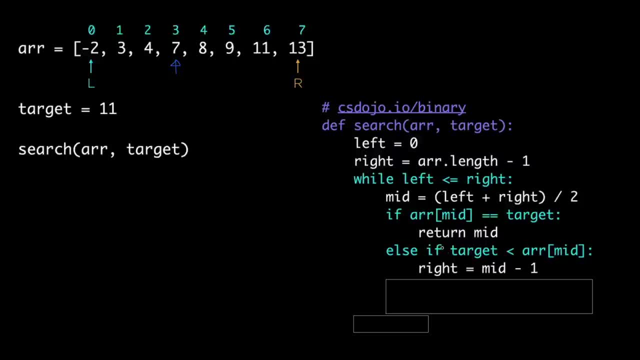 and else if target happens to be less than that element right there. so if the target happens to be, for example, six in this example, then the right pointer will be mid minus one, so the right pointer will move right there and otherwise target is greater than that element right here. 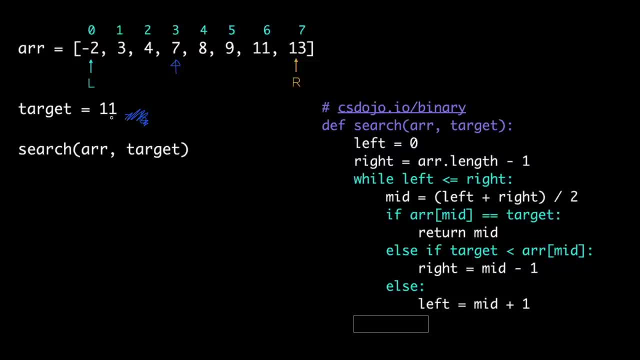 so that's the example we have right here. target happens to be greater than seven, so then left or l will be mid plus one. that's right here. and then we can keep repeating this while loop until we either find r of mid to be target, and at that point we can return mid, or 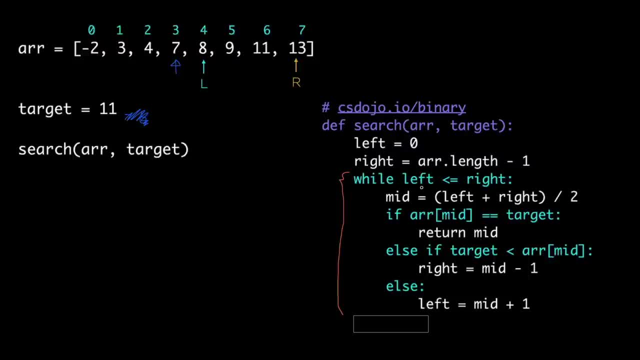 left will be greater than right. so, for example, if the target happens to be, let's say, 12, which doesn't exist in this array, then eventually l will come to the right of r, or in other words, left will be greater than right. so at that point we'll get out of the 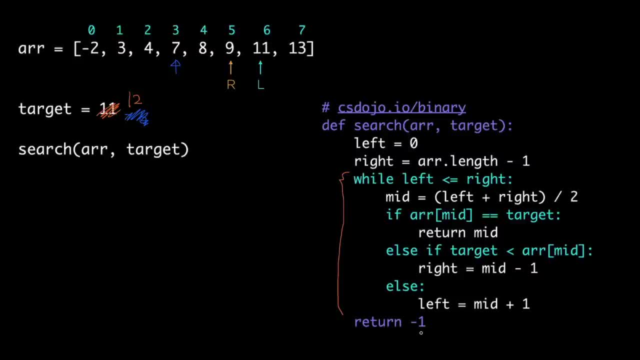 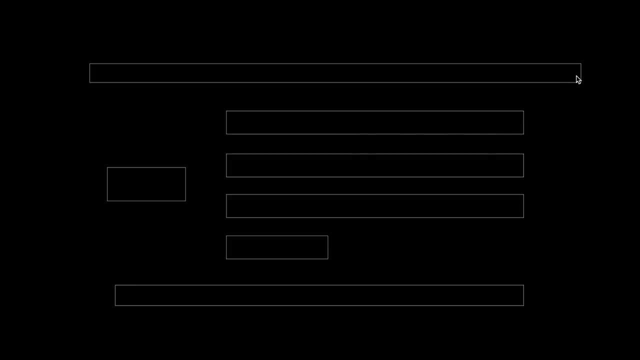 while loop and then we can return minus one to show that the target doesn't exist in this array. okay, so that's how binary search works, but if you're looking for extra practice, i would recommend using my business affiliates product algorexpertio, which you can find at this referral link of mine, and get a discount from. 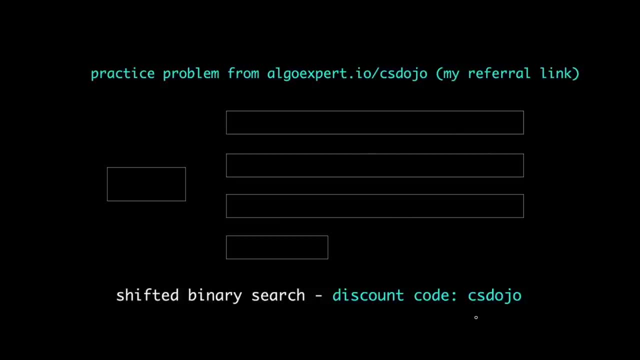 with my discount code csdojo. they have two related problems. one is simply implementing binary search and the second one is called shifted binary search, which i think is much more interesting. so in this problem, you're given a sorted array as well as the target, and you need to find the position of the target. 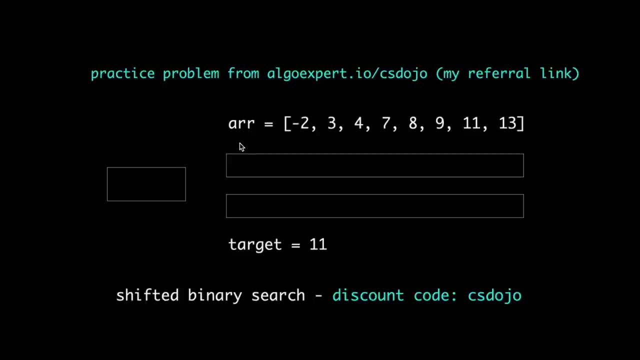 with a little bit of a twist, you could be given a sorted array, just like that. but you could also be given an array that's sorted but also shifted. so if you're given, for example, this array and the target, you can see that it's sorted but shifted by one, just like that, or you could be.